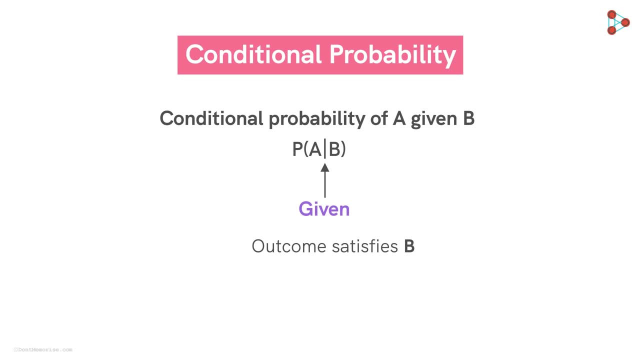 It means, given that the outcome of a random experiment satisfies B, how likely it is that it will also be given? Does this probability also satisfy A? In other words, what are the chances of the occurrence of the event A when, given that the event B has already occurred? 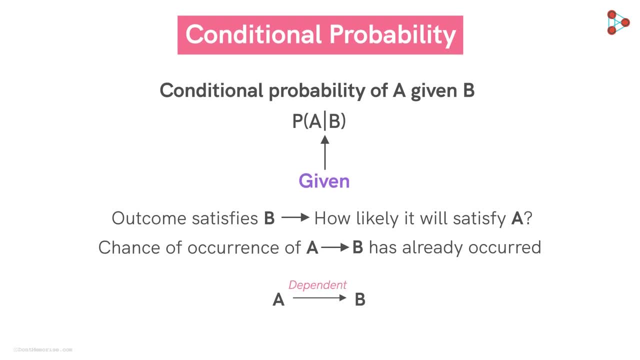 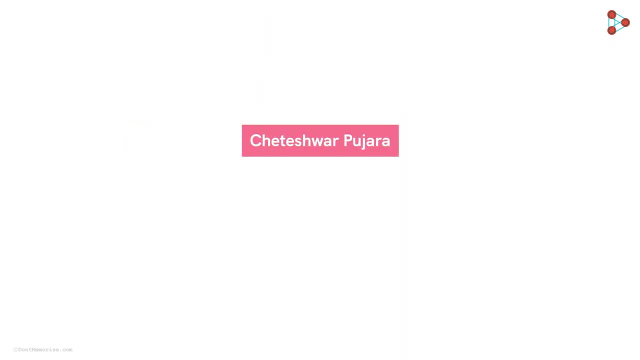 If A and B are dependent events, the knowledge of the occurrence of event B is going to impact the chances of occurrence of event A. Let's understand this using an interesting example. We have Cheteshwar Pujara batting in the air. 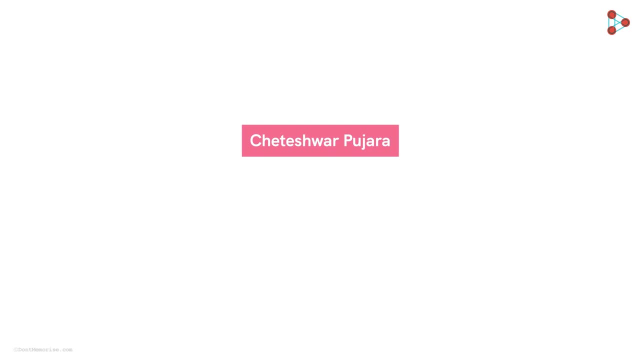 This is the first innings of an international test match. How likely is it that he will score a hundred, given that he has already scored a half century? Now here we have to find the probability that Cheteshwar Pujara will score a hundred in. 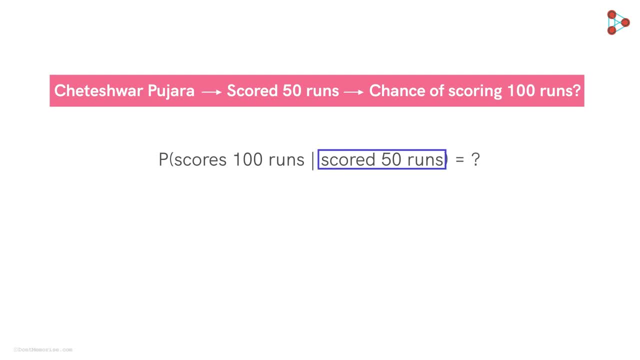 the first innings, given that he has already scored 50 runs. To find this probability, we need some information about his past performances, like how many times has he converted a fifty into a hundred, Or how many times has he converted a fifty into a hundred. 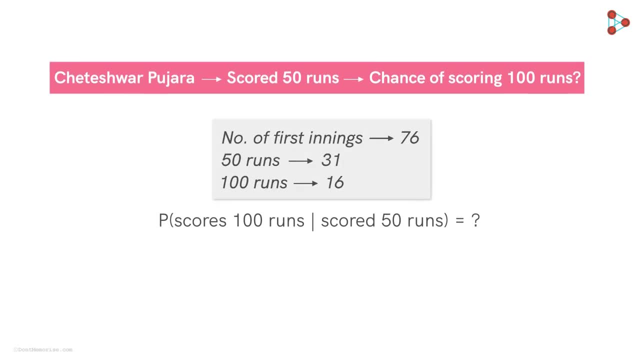 While batting in the first innings. This data is easily available on the internet. Based on our research, it turns out that out of 76 first innings in which he has batted, 31 times he has scored half centuries And 16 out of the 31 times he has gone on to score 100 runs or more. 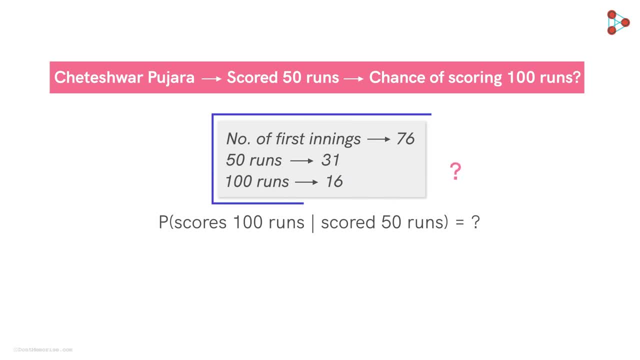 Now, what can we do with this data? This data can help us to predict the likelihood of a hundred. This data can help us to predict the likelihood of a hundred. This data can help us to predict the likelihood of whether he will score a century in the. 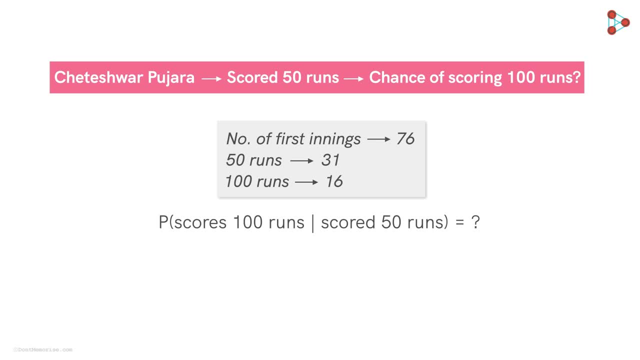 ongoing first innings of a test match after scoring 50 runs. The probability that he will score a hundred or more runs, given that he has scored half a century, will be simply given by 16 by 31.. Where 31 is the total number of times that he had scored a fifty in the first innings. 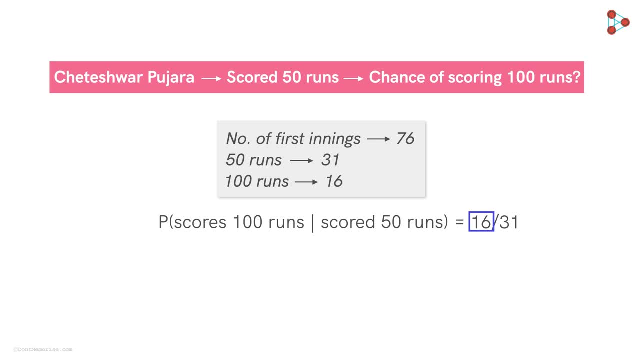 And 16 is the number of times he has converted those fifties into hundreds. The probability that he will score a hundred or more runs, given that he has gone on to score a century, is approximately 12.. Now we should remove from this to now the firstibility of the Probability of Pujara scoring a hundred. 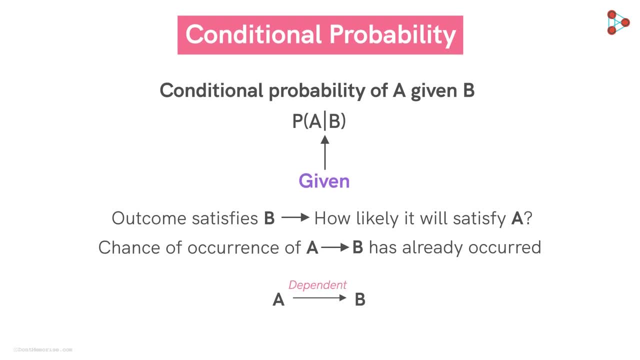 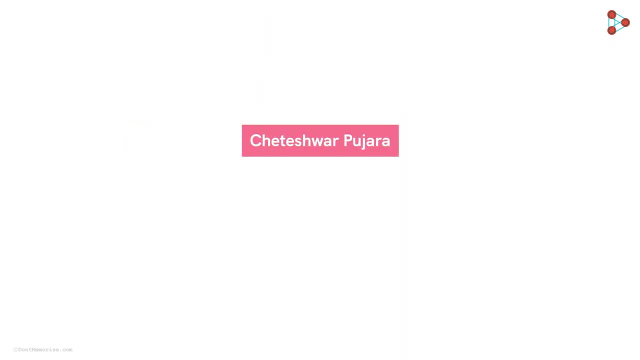 If A and B are dependent events, the knowledge of the occurrence of event B is going to impact the chances of occurrence of event A. Let's understand this using an interesting example. We have Cheteshwar Pujara batting in the air. 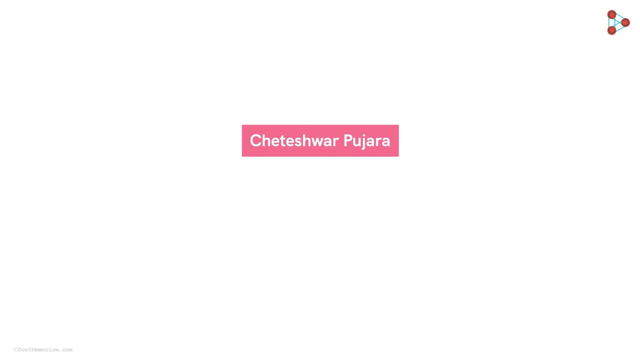 He will score a hundred in the first innings of an international test match. How likely is it that he will score a hundred, given that he has already scored a half-century? Now, here we have to find the probability that Cheteshwar Pujara will score a hundred. 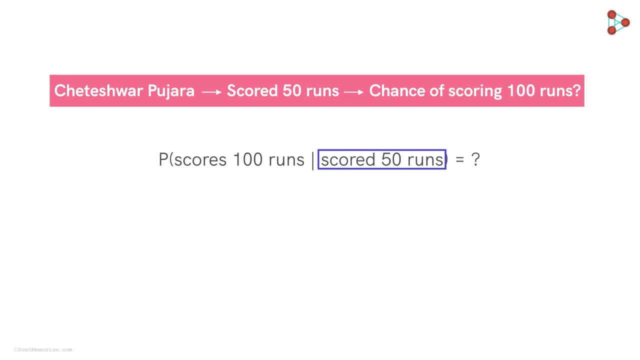 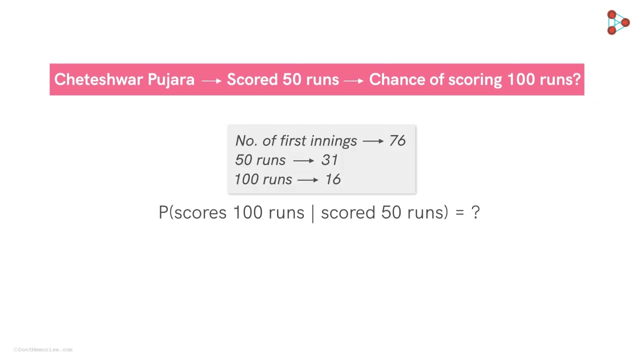 in the first innings, given that he has already scored 50 runs. To find this probability, we need some information about his past performances, like how many times has he converted a fifty into a hundred while batting in the first innings? This data is easily available on the internet. 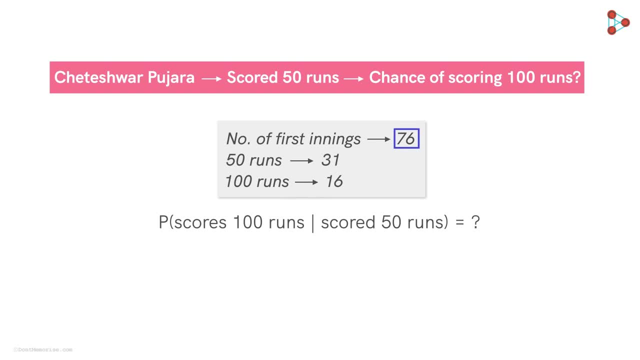 Based on our research, it turns out that, out of 76 first innings in which he's batted 31 times, he's scored half centuries And 16 out of the 31 times he's gone on to score 100 runs or more. 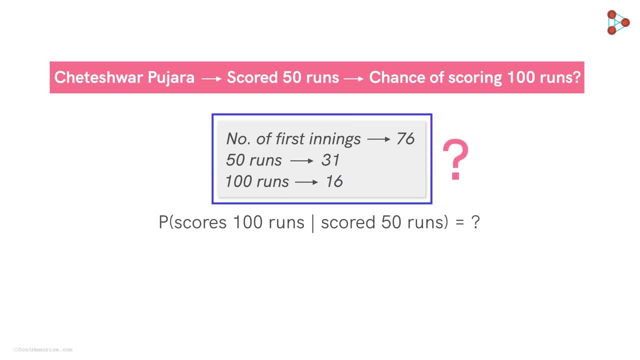 Now what can we do with this data? This data can help us to predict the likelihood of whether he will score a century in the ongoing first innings of a test match. after scoring 50 runs. The probability that he will score 100 or more runs. 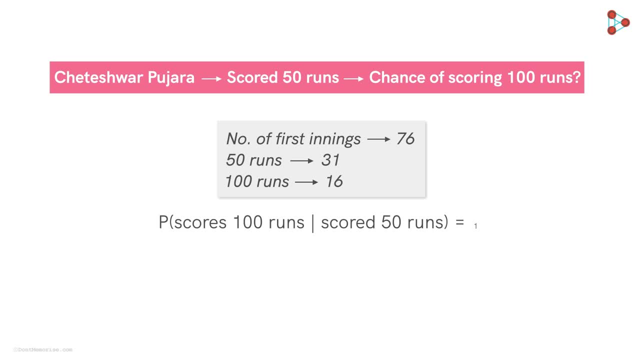 given that he's scored half a century will be simply given by 16 by 31.. Where 31 is the total number of times that he'd scored a 50 in the first innings And 16 is the number of times he's converted. 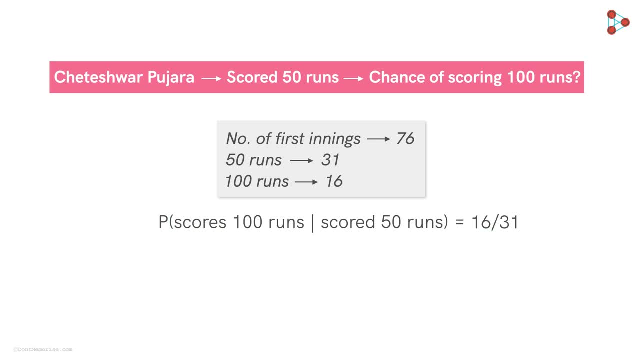 those 50s into 100s, The probability is approximately equal to 52%. Now, the probability of Pujara scoring 100, given that he has scored 50 in the first innings, is not equal to the probability of Pujara scoring 100 in the first innings. 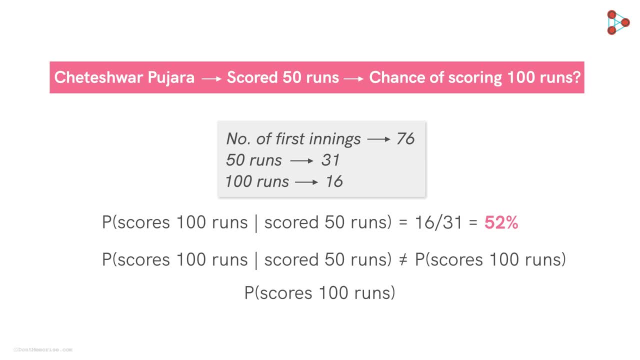 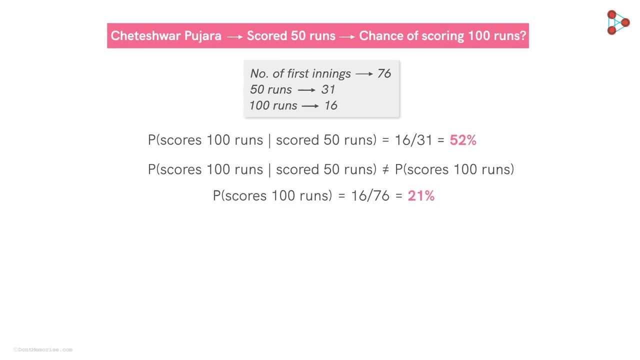 The probability of Pujara scoring 100 in the first innings is given by 16 by 76, which is 21%. Thus we can see that both these probabilities are different. Now let's see if we can represent this mathematically.